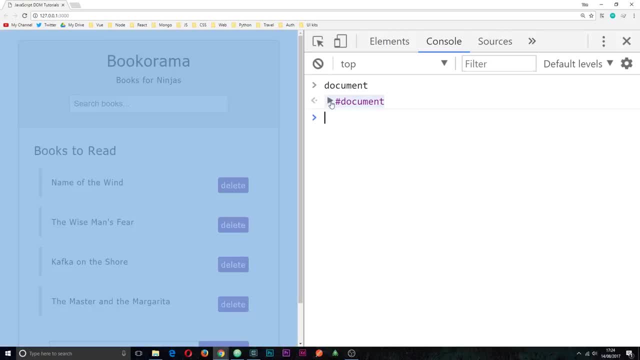 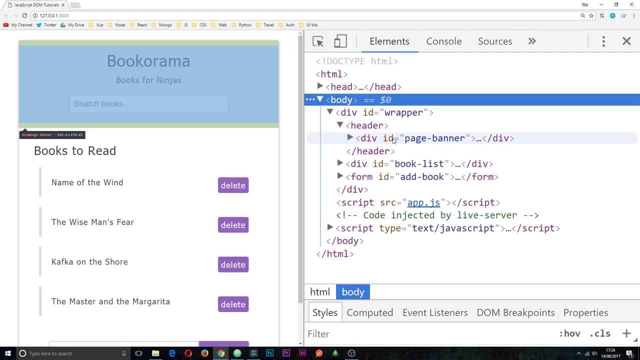 be sitting on this document object. Okay, so I'm going to show you in this tutorial how to reach in and grab an element using an ID, So hopefully you know all about IDs. IDs are an attribute that we give to HTML elements to identify it, if you like, and we can use those IDs in JavaScript to 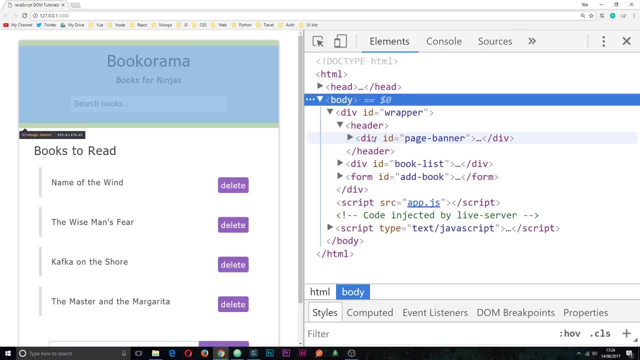 reach in and grab those elements. So, for example, this div right here at the top is going to be an ID of page banner. This one has an ID of book list and this one of add book. Now, typically- not typically, in fact, in all cases- you only want to have one unique ID on each web page. So, for example, 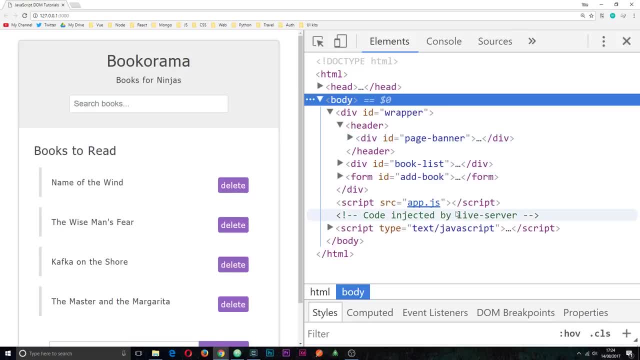 I wouldn't have this ID of page banner and then another banner down here which also has the ID of page banner. These IDs must be unique and associated to only one HTML element. Otherwise, some of these different methods that we use might not be the same as the ones that we use in JavaScript. So 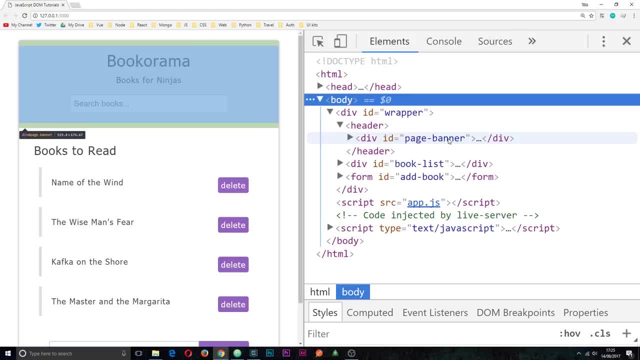 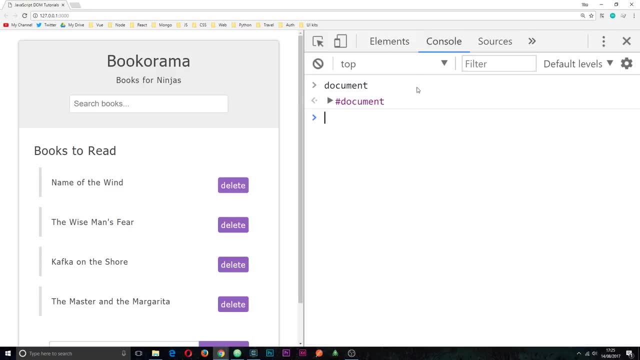 you might throw up results you're not expecting. Okay, so let's go in and grab this element, first of all, This ID of page banner. How do we do that? Well, first of all we say documents and then we're going to use a method on this document object called getElementsByID. So to use a method, dot. 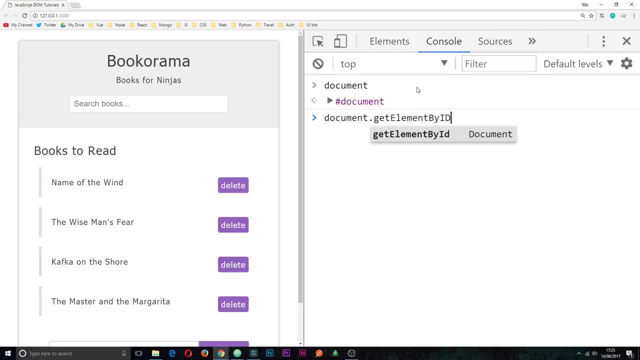 first of all, then getElementsByID, and notice the camel case in here. Each word starts with a capital, except the first one. All right, This method takes in a parameter in these parentheses, and that's going to be the ID that we want. Now we 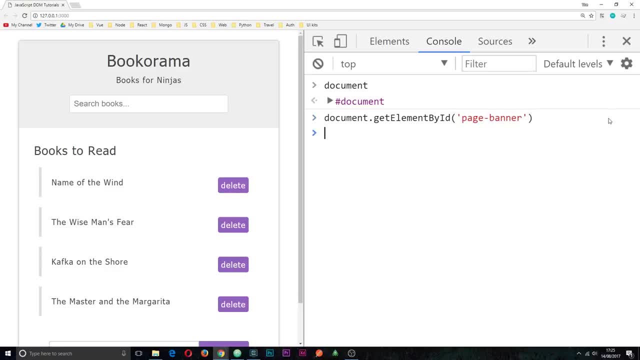 want the ID page hyphen banner. So if I click enter now, what it's going to do is return to us this element. And now we've reached in and we've grabbed that node. So later on I want to show you how we can change this node, How we can change the text content or the HTML. We're going to do this first. 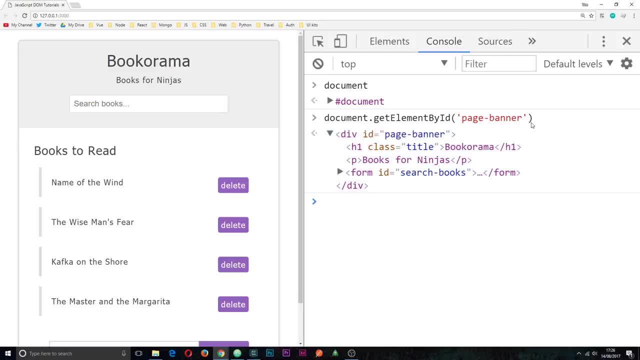 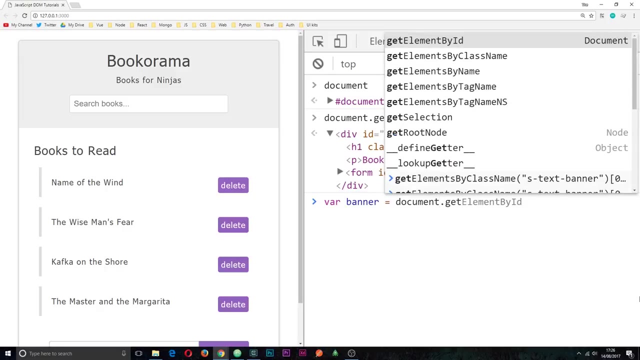 of all. Okay. So this is just one way of reaching in and grabbing an element from the document And we can change the variables if we want to use them at a later time. For example, I could say: var banner is equal to document dot getElementsByID And then inside here we can pass in the page hyphen.